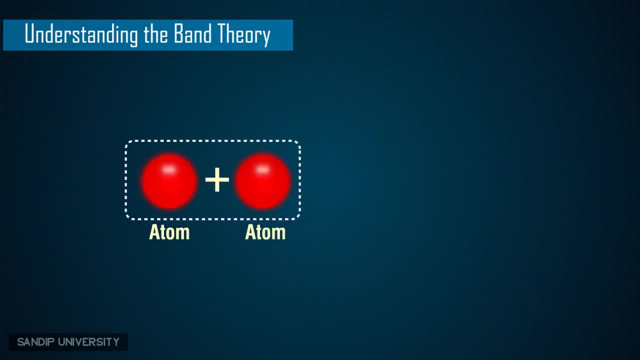 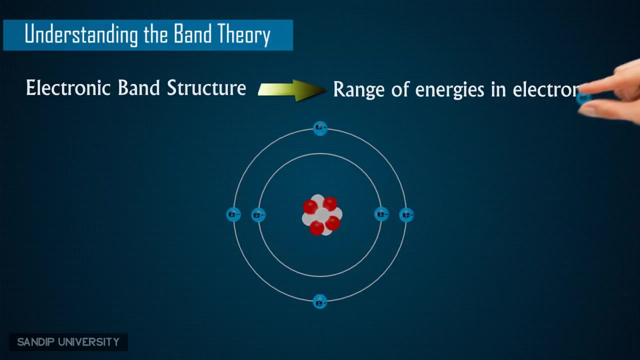 When atoms come together to form a compound, their atomic orbital energies mix together to form molecular orbital energies. The electronic band structure of a matter describes the range of energies that an electron within the matter may have and ranges of energy that it may not have. 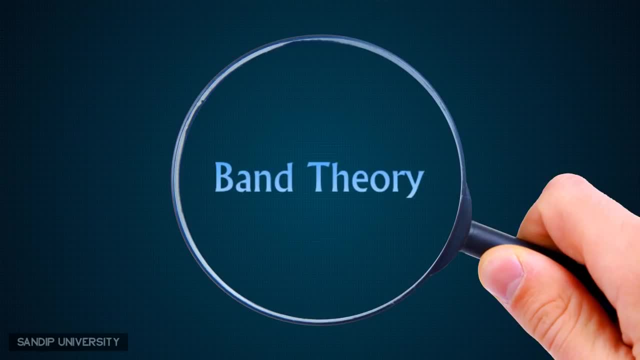 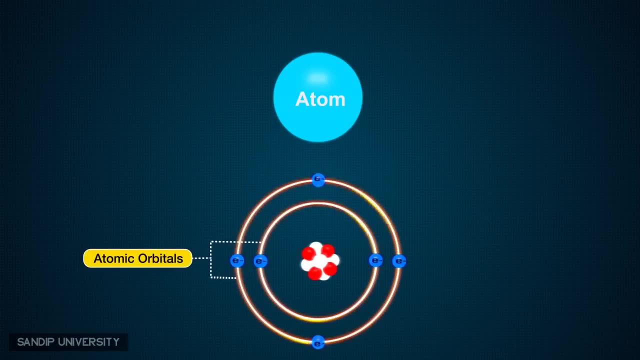 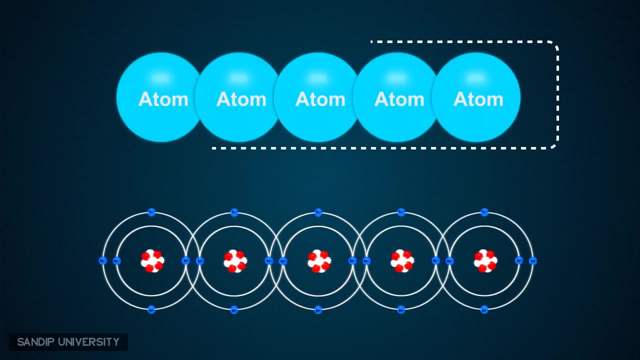 Now let's take a dip into the band theory to understand it further. The electrons of a single isolated energy atom occupy atomic orbitals. Each orbital forms a discrete energy level. When multiple atoms join together to form into a molecule, their atomic orbitals combine to form molecular orbitals. 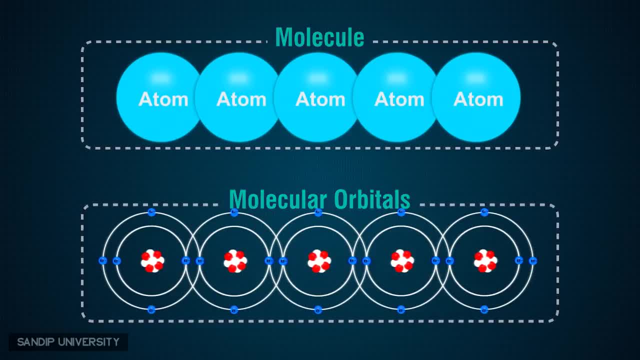 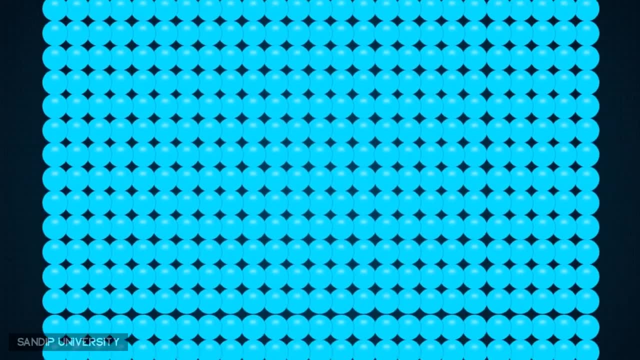 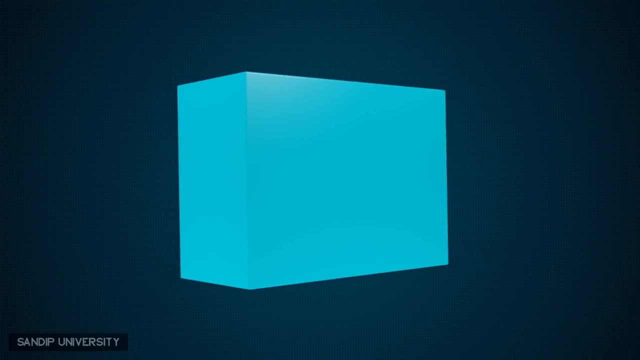 each of which forms at a discrete energy level. As more atoms are brought together, the molecular orbitals extend larger and larger, and the energy levels of the molecule will become increasingly dense. Eventually, the collection of atoms form a giant molecule, or in other words a solid. 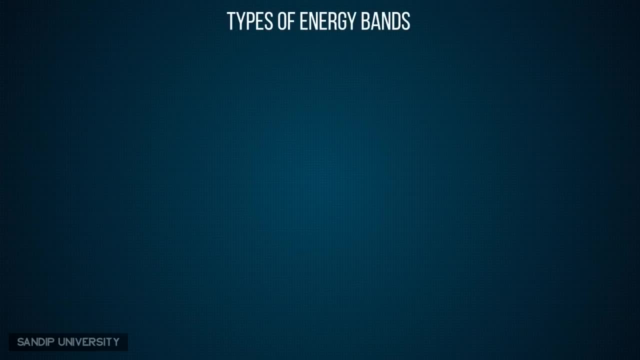 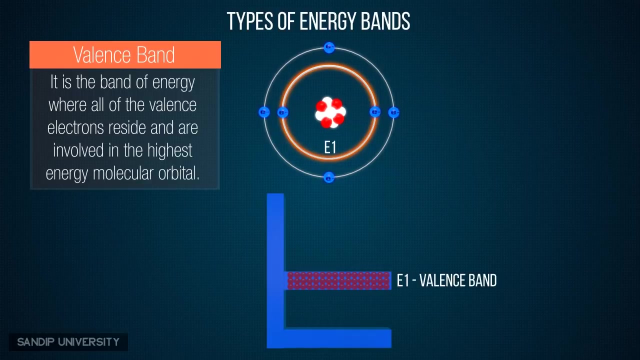 Types of Energy Bands. Let's take a look at various types of energy bands. The first one is valence band. It is the band of energy where all the valence electrons reside and are involved in the highest energy, molecular orbital. And the second one is conduction band. 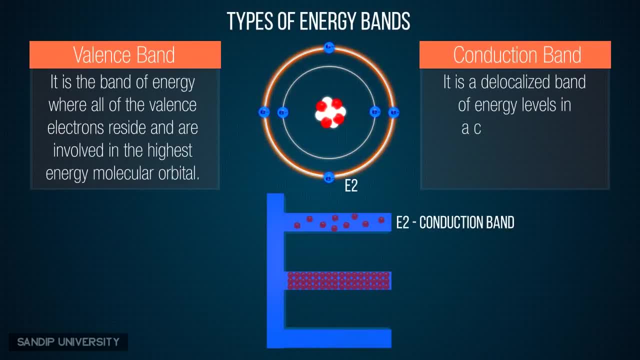 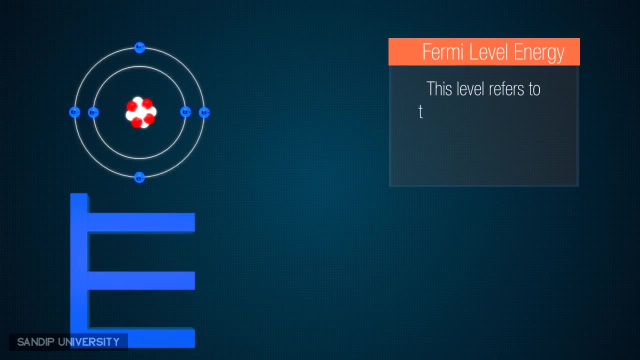 It is a delocalised band of energy levels in a crystalline solid which is partly filled with electrons. These have some great mobility and are responsible for electrical conductivity. Fermi-level energy: This level refers to the highest occupied molecular orbital at absolute zero. 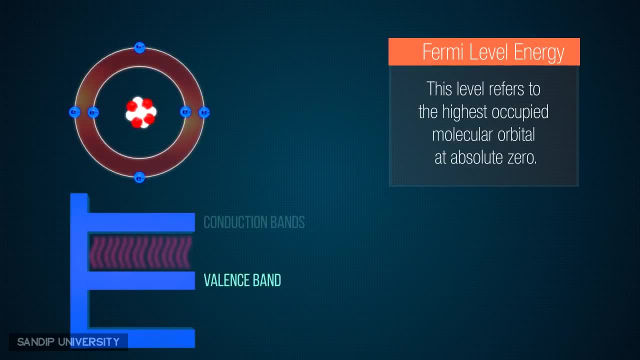 It is usually found at the centre between the valence and conduction bands. The particles in that state have their own quantum states states and generally do not interact with each other. when the temperature begins to rise above absolute zero, these particles will start moving upwards and 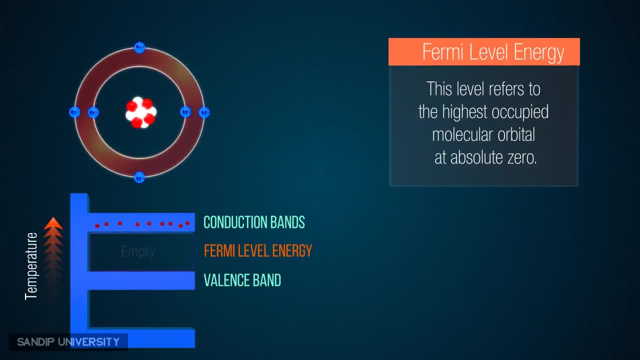 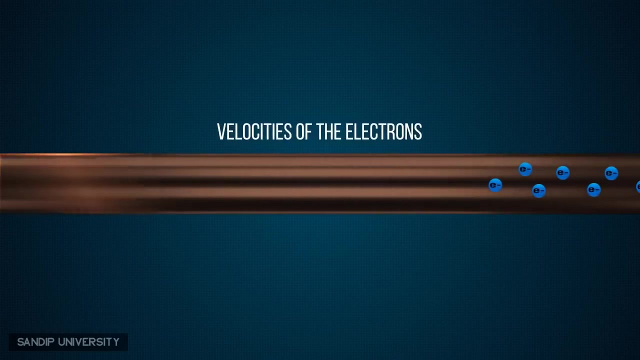 the states below the Fermi level becomes unoccupied. it's pretty much the same thing which you might have inferred, but let me reiterate here for you. in metals, the Fermi energy gives us information about the velocities of the electrons which participate in the ordinary electrical conduction, the amount of